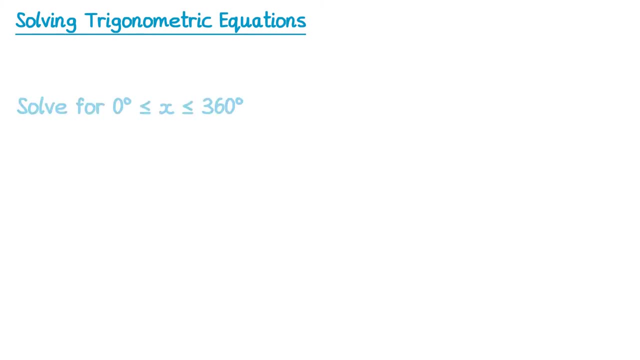 try afterwards. So let's imagine we were going to solve for x values in between 0 and 360 degrees an equation which says cos x equals 0.8. Now based on your knowledge from GCSE maths you should already know that you could inverse cos both sides of this equation and you'll get x 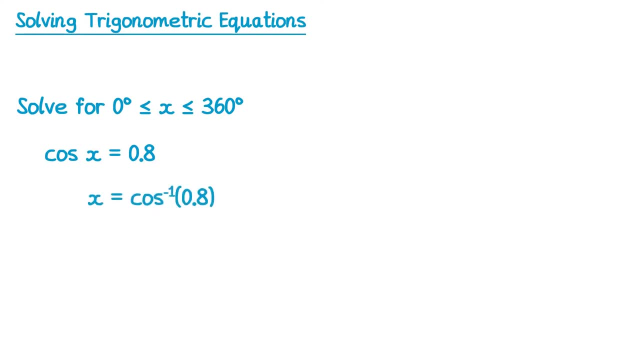 equals inverse cos of 0.8. You can then type this into your calculator and it will give you the answer x equals 36.9 degrees which I've rounded off to one decimal place. So that is one solution to the equation is certainly between 0 and 360 degrees. However it isn't the only solution to this equation. To find the other solution we're going to look carefully at the graph of y equals 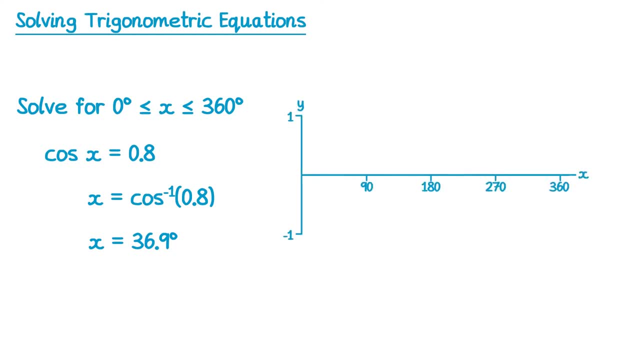 cos of x. So if we draw some axes like this the graph of y equals cos of x starts up here at 1 then it comes down to 0 at 90, negative 1 at 180, back to 0 at 270 and then back at 1 at 360. 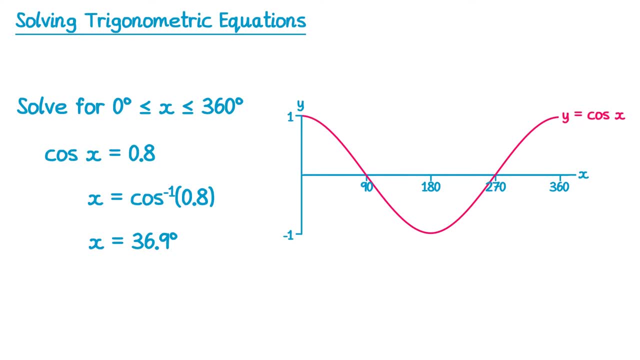 This is the graph of y equals cos of x. Now our equation was when cos of x equals 0.8. So let's mark on 0.8 on the y-axis and see where this function gives us an output value of 0.8. To do this we just draw a horizontal line at 0.8 and you can see there are two intersections. The first of those is the one we've already found. You can see it's less than 90 and bigger than 0 so there's our 36.9 degrees. The question is what is this other solution on the right hand side? To find this we use the symmetry of the cos graph. The cos graph is symmetrical about 180 degrees. You can imagine there's a mirror line down the middle of this graph. This means this distance here is the distance between the cos and the y-axis. So the distance here from 0 to 36.9 degrees must be the same distance from 360 back to our solution. 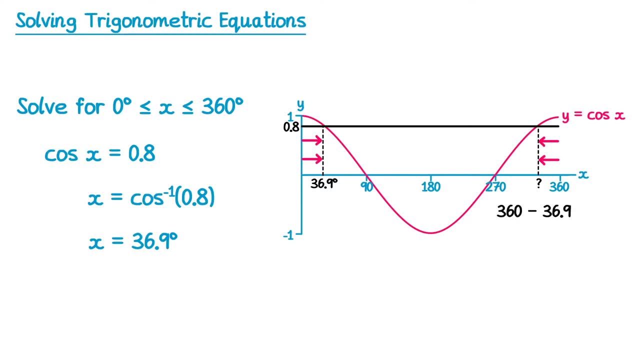 So we can just do 360 take away 36.9 and we found the other solution which is 323.1 degrees. This is also between 0 and 360 so it's a valid solution so we get two solutions to this equation 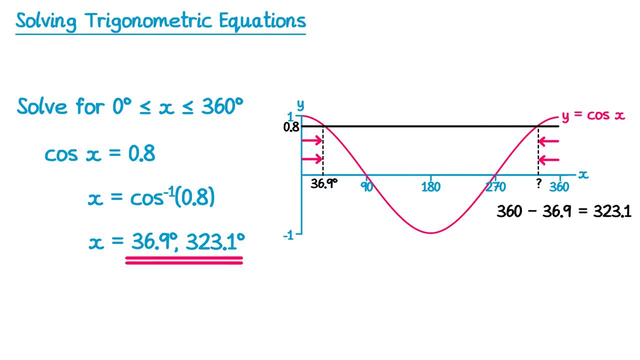 36.9 degrees and also 323.1 degrees. Let's have a look at a second one. So this 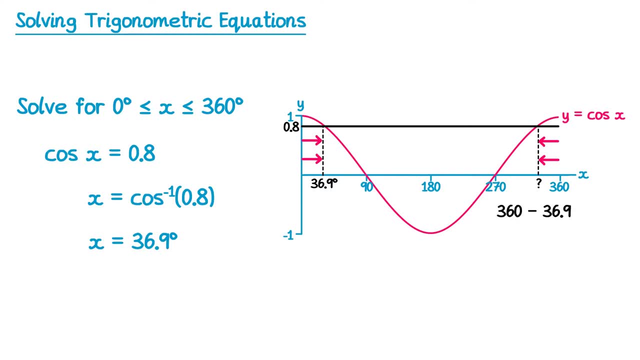 So we can just do 360, take away 36.9, and we found the other solution, which is 323.1 degrees. This is also between 0 and 360, so it's a valid solution. so we get two solutions to this equation: 36.9 degrees and also 323.1 degrees. Let's have a look at a second one, So this: 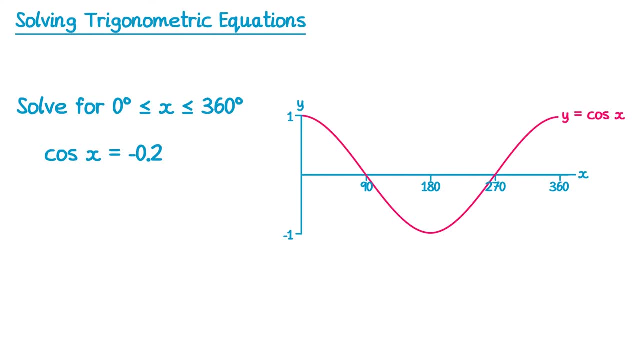 time cos of x equals negative 0.2.. We start just by doing inverse cos of negative 0.2 and with your calculator that gets you 101.5 degrees Again. I'm going to round all of these to one decimal place. Now we mark on to the axes negative 0.2. so that goes about here and draw. 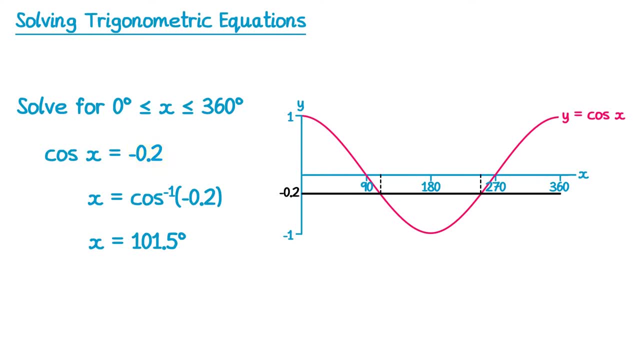 ourselves a horizontal line and you'll see again. there are two intersection points. One of those we have 101.5, that must be this left one here, and we need to find the other one over on the right property of the cos graph. The horizontal distance here from 0 to our solution is 101.5. 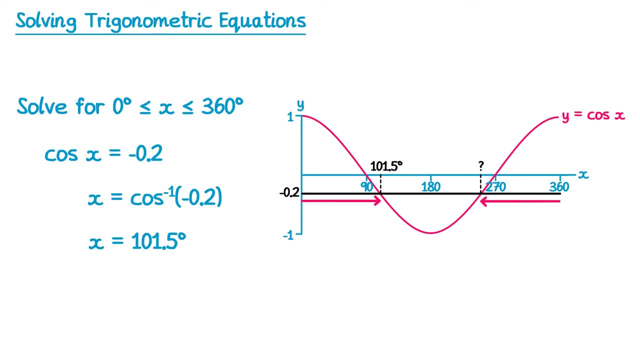 that must be the same distance from 360. back to our second solution. So we do 360, take away 101.5 and we get the other solution, 258.5.. So we have two solutions: 101.5 and 258.5.. 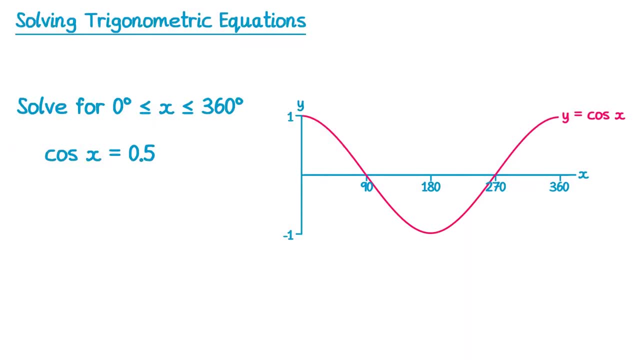 The questions we've looked at so far will be on the calculator paper. however, you could be given questions like this on the calculator paper. So let's start with the calculator paper. This is testing your knowledge of exact values of trig functions. So for this one, we start by doing: 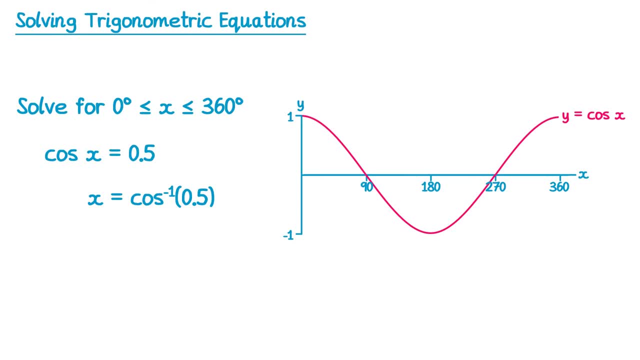 x equals inverse cos of 0.5, but you should already know that inverse cos of 0.5 is 60 degrees, since cos of 60 equals one half. So one of the solutions is 60 degrees. Let's use the graph to find the. 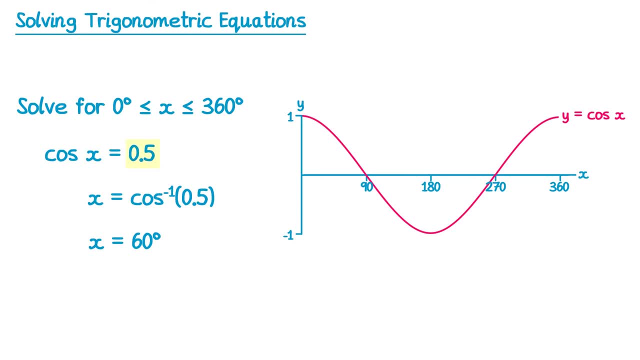 other one. So we're trying to find when cos of x equals 0.5. so we mark 0.5 on the axis, draw on a horizontal line and we'll find the two intersections: The one we've already got, which is 60 degrees, and then there's one over on the right hand side as well. We use the symmetry. 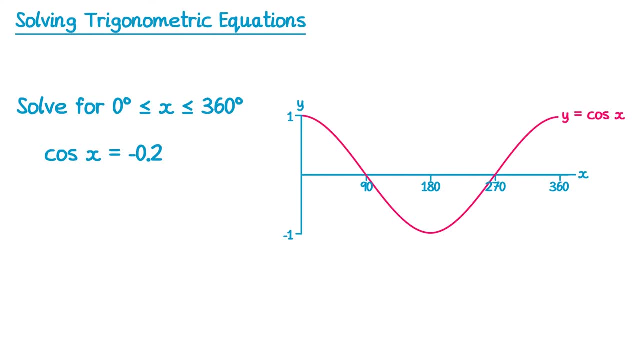 time cos of x equals negative 0.2. We start just by doing inverse cos of negative 0.2 and with your calculator that gets you 101.5 degrees. Again I'm going to round all of these to one decimal place. Now we mark on to the axes negative 0.2 so that goes about here and draw 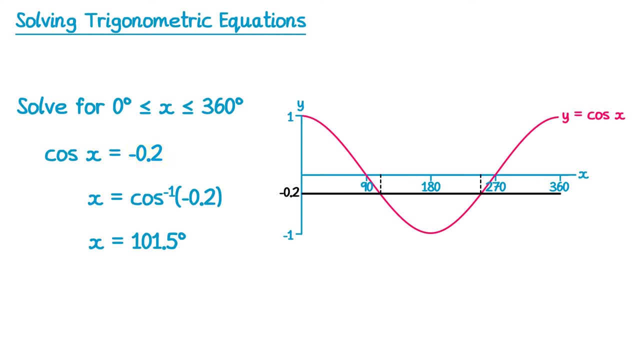 ourselves a horizontal line and you'll see again there are two intersection points. One of those we have 101.5 that must be this left one here and we need to find the other one over on the right 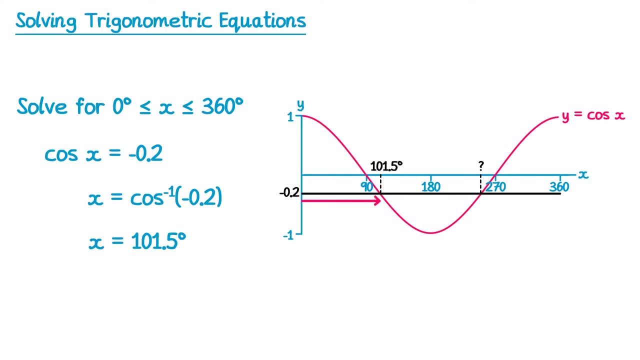 property of the cos graph. The horizontal distance here from 0 to our solution is 101.5 that must be the same distance from 360 back to our second solution. So we do 360 take away 101.5 and we get the other solution 258.5. So we have two solutions 101.5 and 258.5. 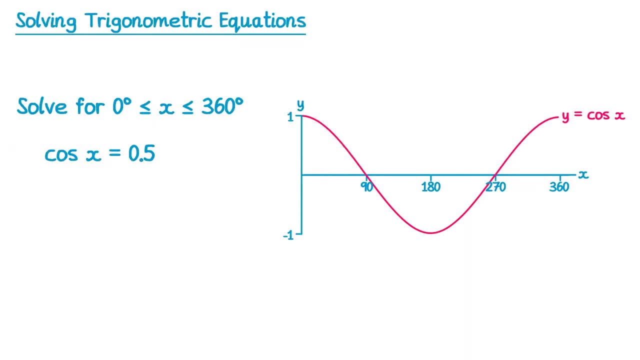 The questions we've looked at so far will be on the calculator paper however you could be given 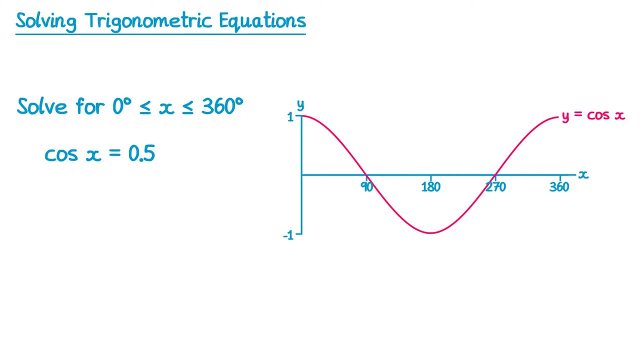 questions like this on the calculator paper. So let's start with the calculator paper. This is testing your knowledge of exact values of trig functions. So for this one we start by doing x equals inverse cos of 0.5 but you should already know that inverse cos of 0.5 is 60 degrees since cos of 60 equals one half. So one of the solutions is 60 degrees. Let's use the graph to find the other one. So we're trying to find when cos of x equals 0.5 so we mark 0.5 on the axis, draw on a horizontal line and we'll find the two intersections. The one we've already got, which is 60 degrees and then there's one over on the right hand side as well. We use the symmetry of the graph so from 0 to 60 here is 60 degrees. That must be the same distance from 360 back to our solution. So 360 take away 60 is 300 degrees. So we have two solutions 60 degrees and 300 degrees. Remember this one you'd need to be able to do completely without a calculator. 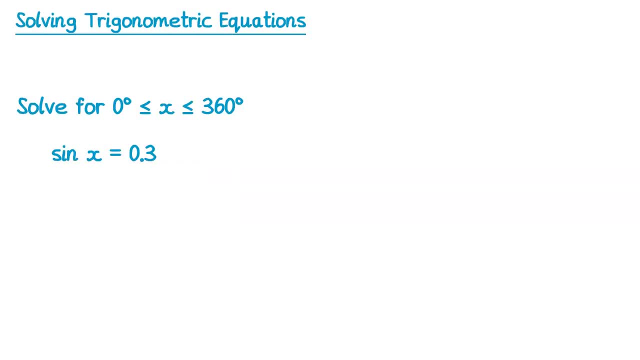 Now let's look at some equations with sine. Well you'd start in the same way so inverse sine of 0.3 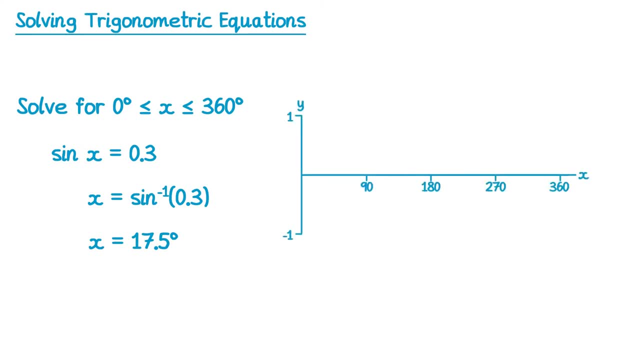 gives you 17.5 to one decimal place and now let's draw the graph of sine of x. So sine of x starts at 0, it goes up to 1 at 90, back down to 0 at 180, then down to negative 1 at 270 and back to 0 at 360. 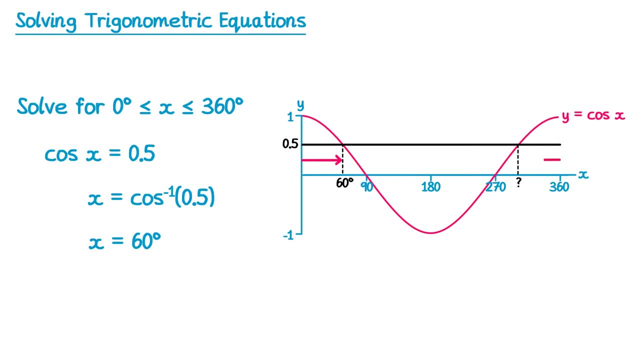 of the graph. so from 0 to 60, here is 60 degrees. That must be the same distance. from 360 back to our solution. So 360 take away 60 is 300 degrees. So we have two solutions: 60 degrees and 300. 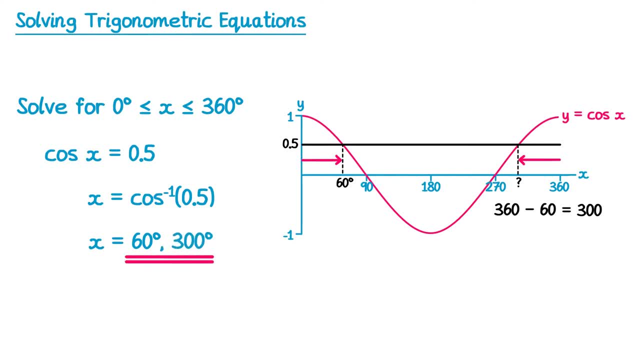 degrees. Remember this one you'd need to be able to do completely without a calculator. Now let's look at some equations with sine. Well, you'd start in the same way. so inverse sine of 0.3 gives you 17.5 to one decimal place. and now let's draw the graph of sine of x. So sine of x starts at. 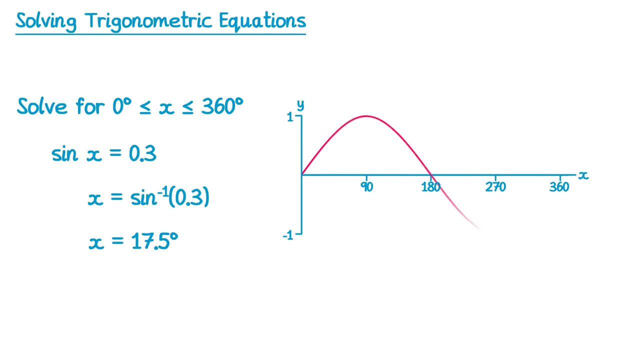 0, it goes up to 1 at 90, back down to 0 at 180, then down to negative 1 at 270 and back to 0 at 360.. So this is the graph. of y equals sine x. Now we'll do the same thing as we did before, so we're. 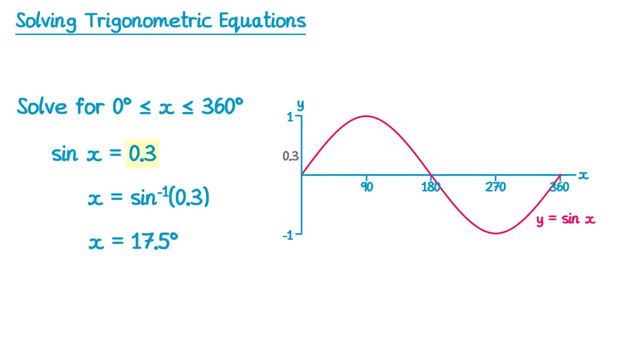 trying to find sine. x equals 0.3, so let's mark 0.3 on the y-axis. Now we draw a horizontal line and we find there are two intersections. again, We can already see one of those, that's our 17.5. 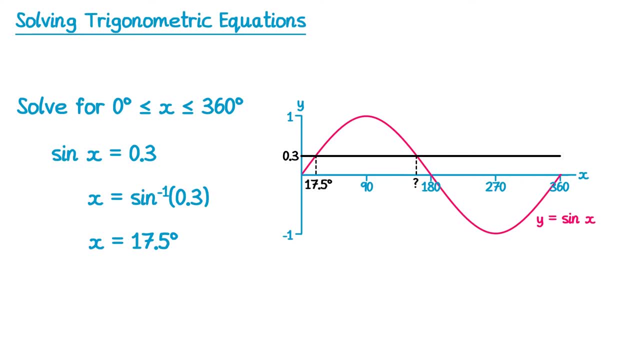 on the left, but what's this solution over here on the right? Now? the symmetry of the sine graph is different to the cos graph. The line of symmetry would be at 90 degrees. So this time we're looking for this horizontal distance here, from 0 to 17.5 is the same as the horizontal 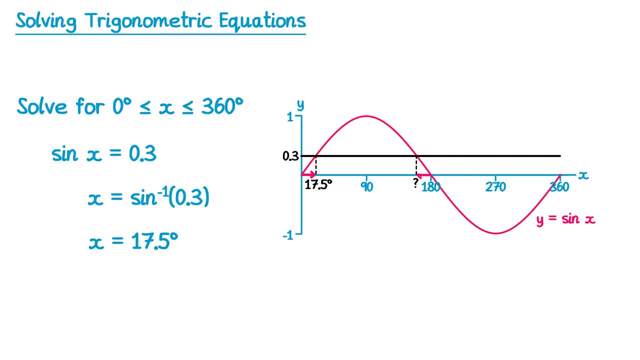 distance from 180 back to our solution. So it's not 360 this time. So to find the other solution, we do 180, take away 17.5 and that gives you 162.5.. So we have two solutions: 17.5 and one. 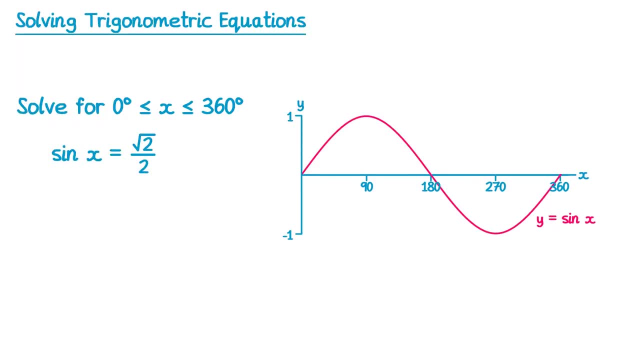 162.5.. This is another example of sine. Again, this would be a non-calculator question. So do inverse sine of square root 2 over 2.. You should know that this is 45, since sine of 45 is square root 2 over 2.. So for this equation we were finding sine x equals root 2 over 2.. We can mark. 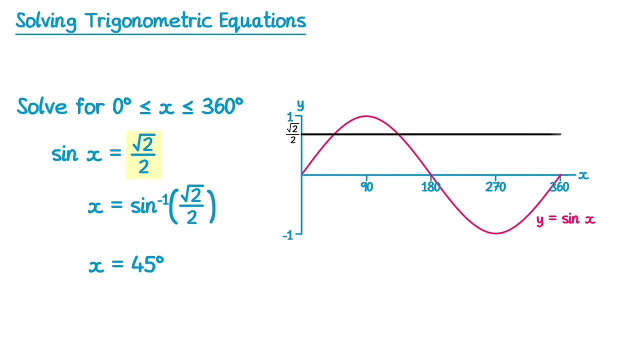 that on our axis here and draw on a horizontal line and we get two solutions. The first of those is 45. we know that one and we have this second one over on the right hand side. 0 to 45 is 45 degrees. That must be the same distance from 180 back to our solution. So we do. 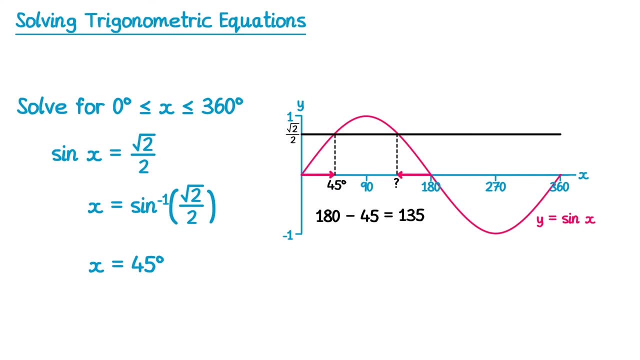 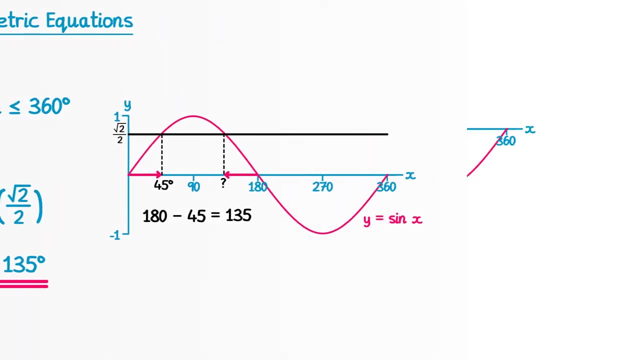 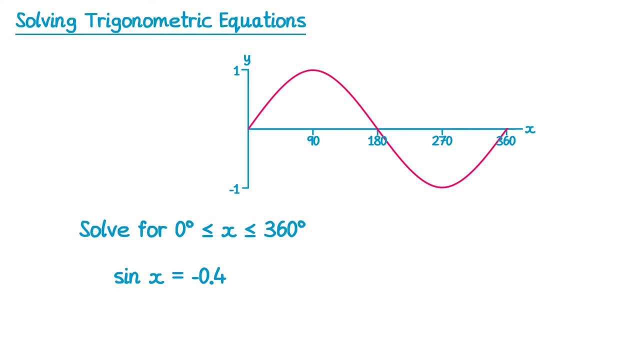 180. take away 45, which is 135.. So you get two solutions: 45 and 135. And again, this one would be non-calculator. Now this is where things get a little bit tricky. When you're solving an equation with sine but equal to a negative value, something different happens. So let's go ahead and do. 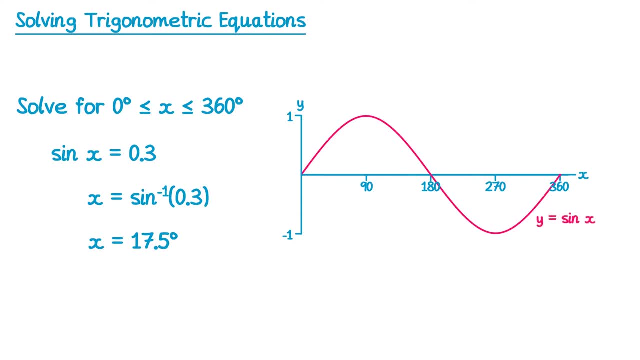 So this is the graph of y equals sine x. Now we'll do the same thing as we did before, so we're trying to find sine x equals 0.3 so let's mark 0.3 on the y-axis. Now we draw a horizontal line and we find there are two intersections again. We can already see one of those that's our 17.5, on the left but what's this solution over here on the right? Now the symmetry of the sine graph is different to the cos graph. The line of symmetry would be at 90 degrees. So this time we're looking for this horizontal distance here from 0 to 17.5 is the same as the horizontal distance from 180 back to our solution. So it's not 360 this time. So to find the other solution 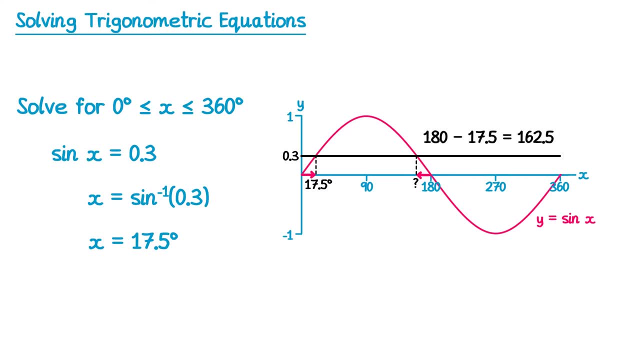 we do 180 take away 17.5 and that gives you 162.5. So we have two solutions 17.5 and one 162.5. This is another example of sine. Again this would be a non-calculator question. 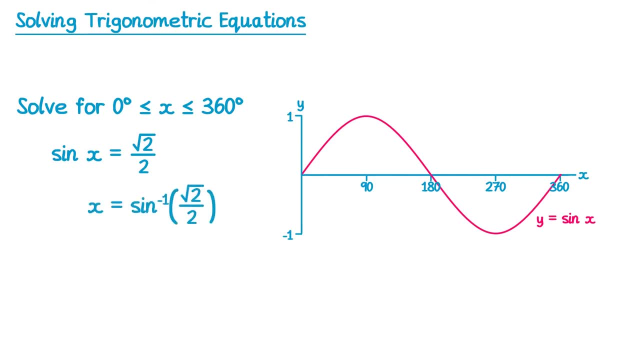 So do inverse sine of square root 2 over 2. You should know that this is 45 since sine of 45 is square root 2 over 2. So for this equation we were finding sine x equals root 2 over 2. 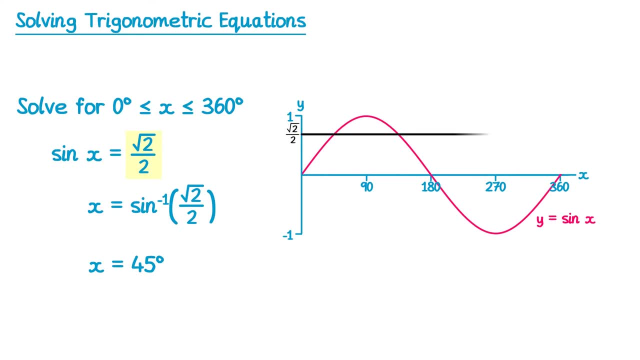 We can mark that on our axis here and draw on a horizontal line and we get two solutions. The first of those is 45 we know that one and we have this second one over on the right hand side. 0 to 45 is 45 degrees. That must be the same distance from 180 back to our solution. So we do 180 take away 45 which is 135. So you get two solutions 45 and 135. And again this one would be non-calculator. Now this is where things get a little bit tricky. 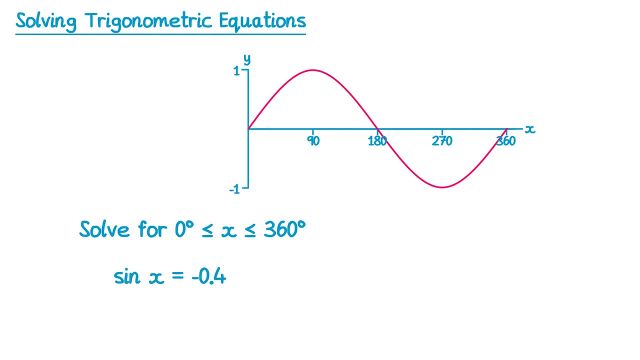 When you're solving an equation with sine but equal to a negative value something different happens. So let's go ahead and do inverse sine of negative 0.4. 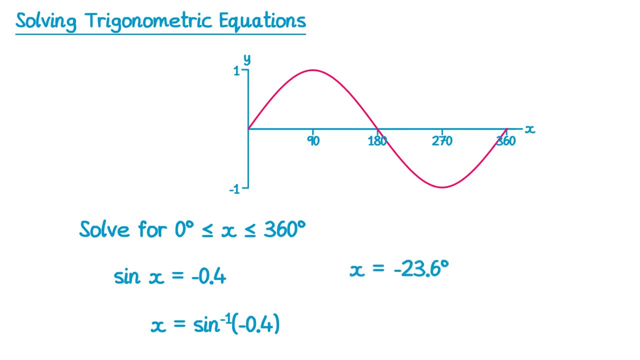 If you type this in the your calculator it will tell you negative 23.6 degrees. Now we need solutions from 0 to 360 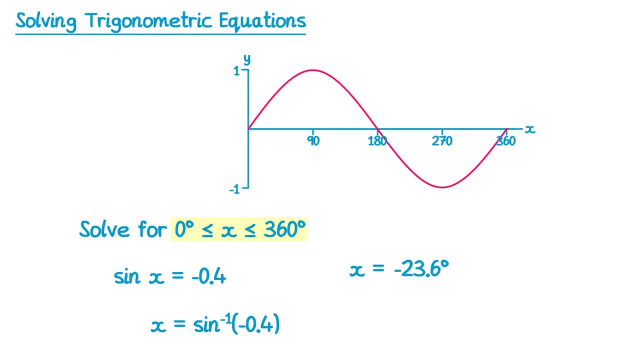 degrees so this solution isn't okay. So what's going on? Well let's draw the usual line onto our graph at negative 0.4. So that would be somewhere like here. We draw that horizontal 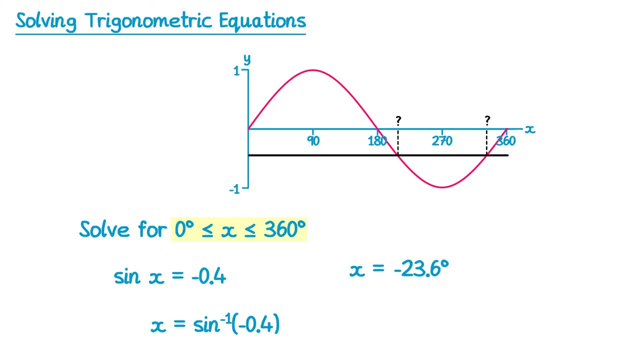 line and we can see the two solutions that we want. However we don't have either of those solutions at 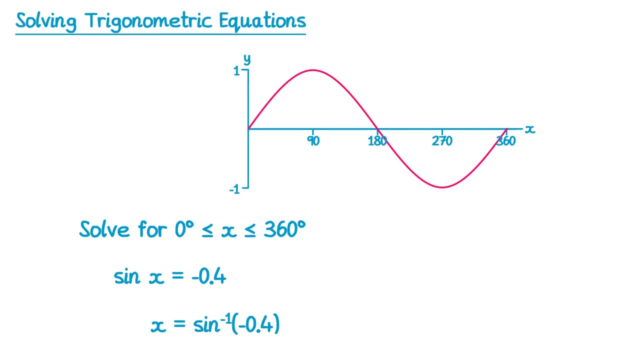 inverse sine of negative 0.4.. If you type this in your calculator, it will tell you negative 23.6 degrees. Now we need solutions from 0 to 360 degrees. So this solution isn't okay. So what's going on? Well, let's draw the usual line onto. 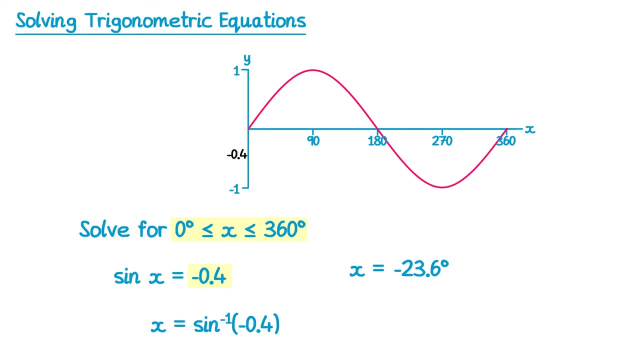 our graph at negative 0.4.. So that would be somewhere like: here We draw that horizontal line and we can see the two solutions that we want. However, we don't have either of those solutions at the minute. We have negative 23.6.. So what we're going to do is extend the sine. 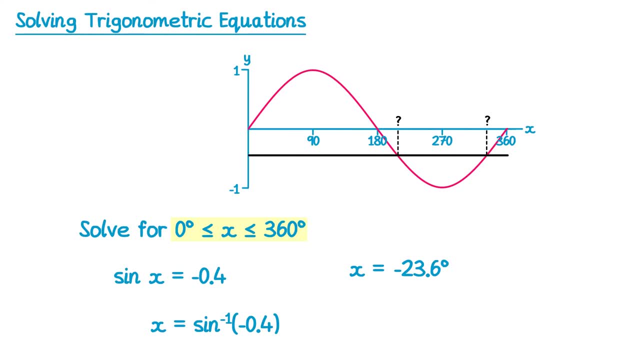 graph backwards. Remember we're going to draw the sine graph backwards, So we're going to remember the trigonometric graphs go on forever and ever in both directions, So let's extend this one backwards. It will continue like this and come back to the axis at negative. 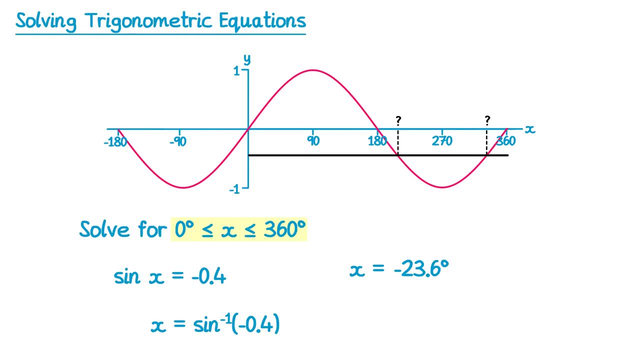 180 degrees. Now let's also extend our black horizontal line and you'll find there are two more solutions. We don't want either of these two solutions because they're not between 0 and 360.. However, one of them is a solution that we have. You can see this one here will. 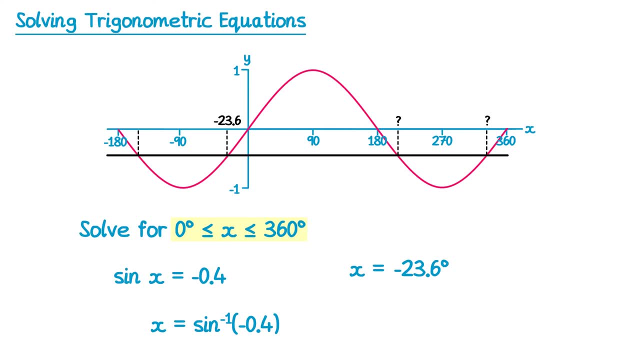 be negative 23.6 degrees. Now, it may not make much sense at this point, but we're going to find the other solution as well, even though it's negative and not in the range we want. We're going to use some symmetry again. So, from here to negative 23.6. 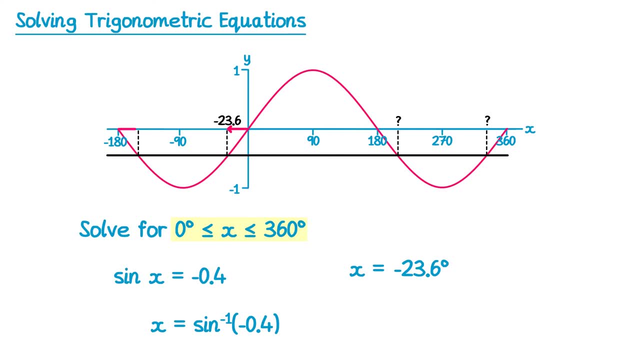 is a distance of 23.6, which must be the same distance from negative 180 to the new solution here. So we do negative 180 plus 23.6 and we find that this solution is negative 156.4.. So we found another solution, not one we want, but we found another one. 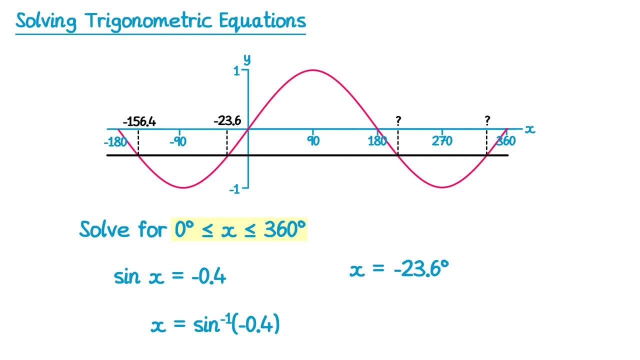 Now there's a really important property of this sine graph. It applies to the cos graph but it repeats every 360 degrees. So to find those solutions that I do want on the right hand side, I'm just going to add 360 degrees to these two solutions that I have. So if 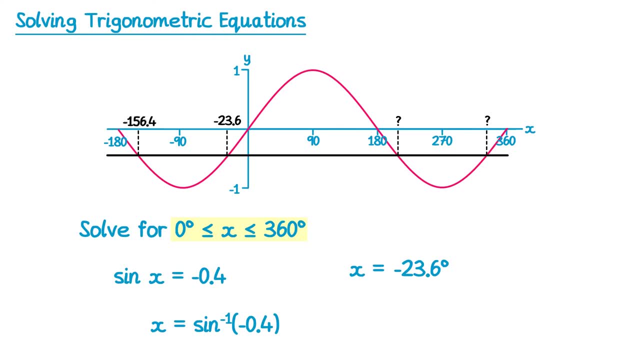 we start with negative 156.4 and add 360 to it. we end up with this solution here at 203.6 degrees. So we did negative 156.4 plus 360, which is 203.6.. And we'll do the same with. 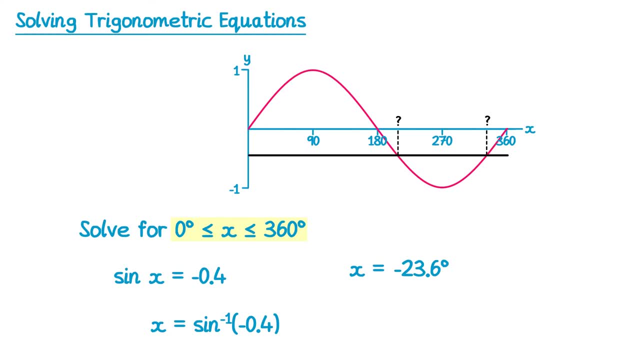 the minute. We have negative 23.6. So what we're going to do is extend the sine graph backwards. Remember the trigonometric graphs go on forever and ever in both directions. So let's extend this 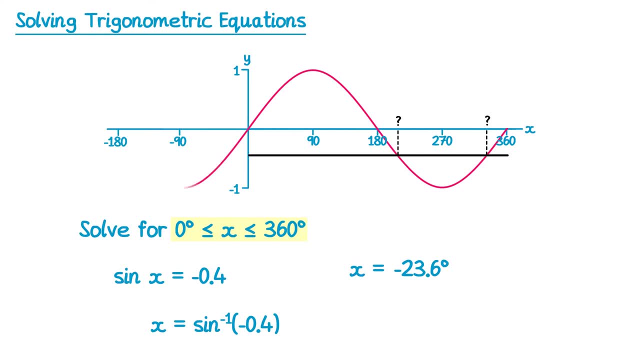 one backwards. It will continue like this and come back to the axis at negative 180 degrees. 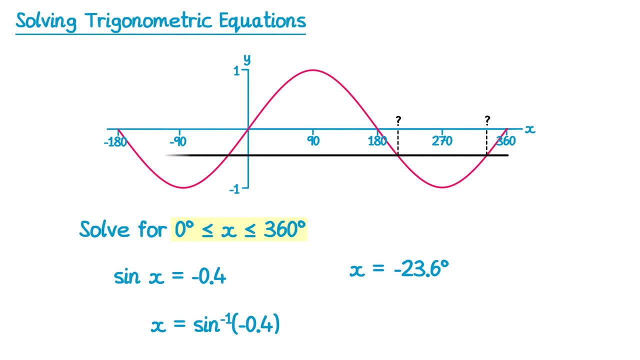 Now let's also extend our black horizontal line and you'll find there are two more solutions. We don't want either of these two solutions because they're not between 0 and 360. However one of them 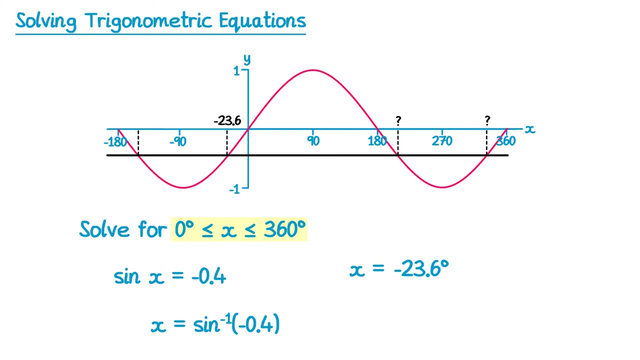 is a solution that we have. You can see this one here will be negative 23.6 degrees. Now it may not make sense at this point but we're going to find the other solution as well even though it's negative 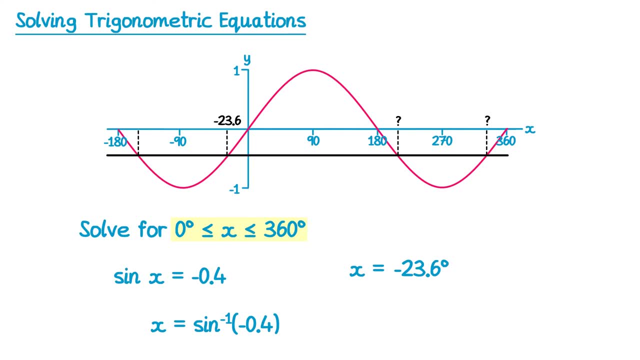 and not in the range we want. We're going to use some symmetry again. So from here to negative 23.6 is a distance of 23.6 which must be the same distance from negative 180 to the new solution here. 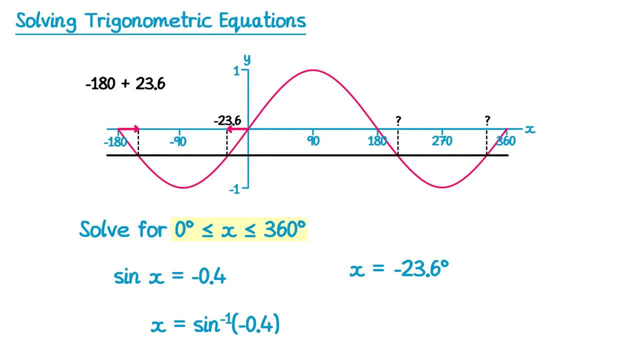 So we do negative 180 plus 23.6 and we find that this solution is negative 156.4. So we found another solution. Not one we want but we found another one. Now there's a really important property of this solution. We'll just add this one to the graph as well but it repeats every 360 degrees. So to find those solutions that I do want on the right hand side I'm just going to add 360 degrees to these two solutions that I have. So if we start with negative 156.4 and add 360 to it we end up with this solution here at 203.6 degrees. So we did negative 156.4 plus 360 which is 203.6 and we'll do the same with the other one. So negative 23.6. Add 360 to it and we get this one. So negative 23.6 plus 360 is 336.4. So we've now found the two solutions we wanted. They're both between 0 and 360 and they are 203.6 degrees and 336.4 degrees. 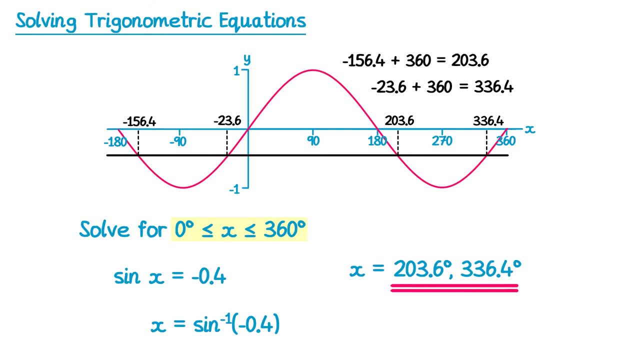 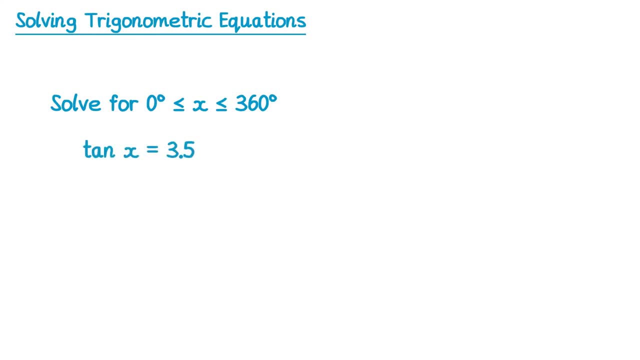 So it's really tricky when you have sine and negative values on the right hand side of the equation. Now what about tan? So we need to look at some tan equations as well. Let's look at 10x equals 3.5. 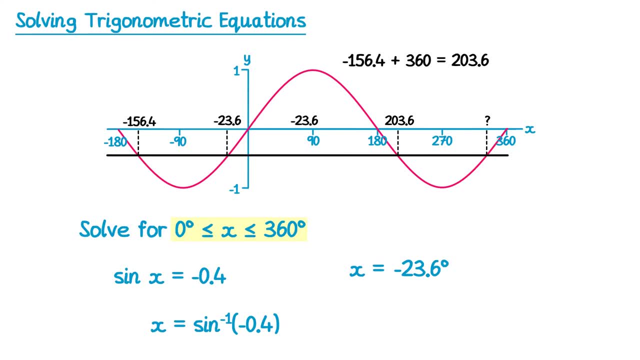 the other one, So negative 23.6,. we add 360 to it, we add 360 to it and we get this one. So negative 23.6 plus 360 is 336.4.. So we've now found the two solutions we wanted. They're both between 0 and 360 and they are. 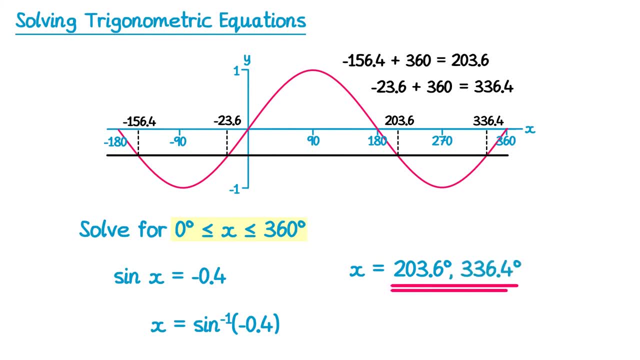 203.6 degrees and 336.4 degrees. So it's really tricky when you have sine and negative values on the right hand side of the equation. Now, what about tan? So we need to look at some tan equations as well. Let's look at: 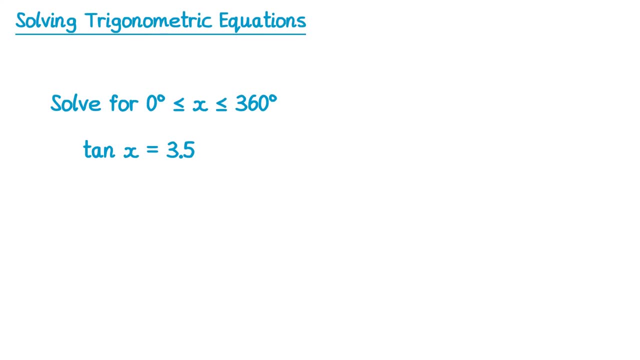 10x equals 3.5.. Say, we do inverse tan of 3.5 and that gives you 74.1 degrees to one decimal place. Now let's draw the graph of y equals tan of x. You should know that there are two asymptotes. 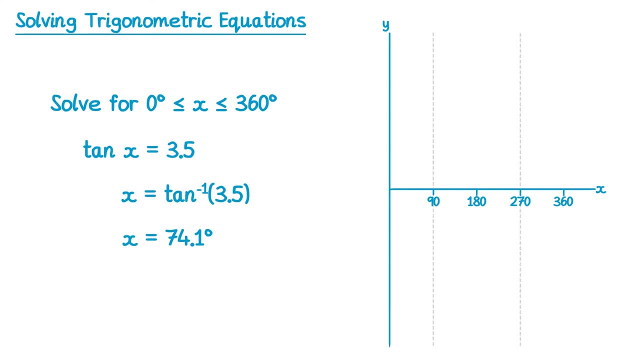 on the graph of tan x You can see those at 90 and 270 degrees And the graph goes like this. So we're trying to solve this equation equal to 3.5.. So we'll draw a horizontal line at 3.5, somewhere about here, and we get two solutions. 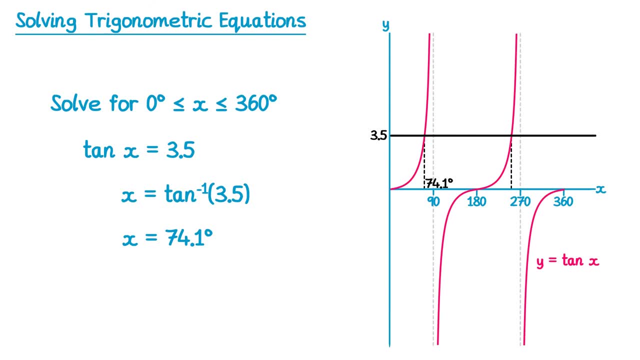 So one of those is our 74.1,. that's going to be the left hand solution here and we need to find the right hand solution Now. tan is actually quite nice because tan repeats every 180, not 360, but 180. So we 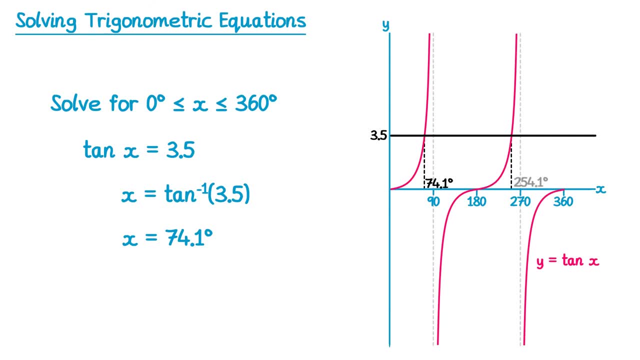 add 180 to 74.1 and we just get the next solution. So 74.1 plus 180 is 254.1.. So there's our two solutions: 74.1 and 254.1 degrees. Now to end the equation with sine. if you make tan equal to a negative value, we do have a. 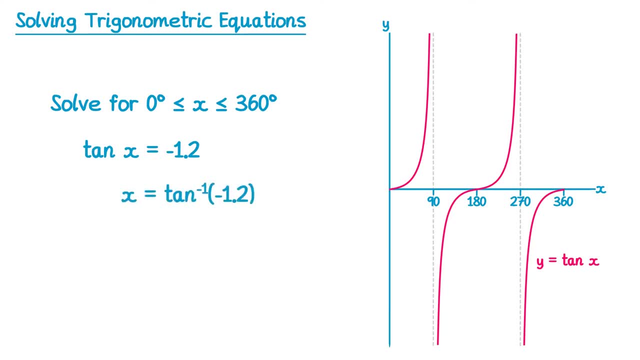 similar problem again. So if we do inverse tan of negative 1.2, we end up with negative 50.2, which isn't in between 0 and 360 degrees. So we need to extend the tan graph backwards as well. 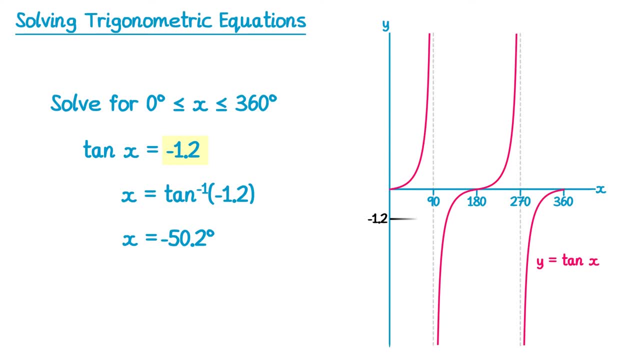 So this one was equal to negative 1.2,. so we'll draw that horizontal line on first And you can see the two solutions that we're trying to find. they're here Now. if we extend the graph backwards, we'll have another asymptote at negative 90 degrees. 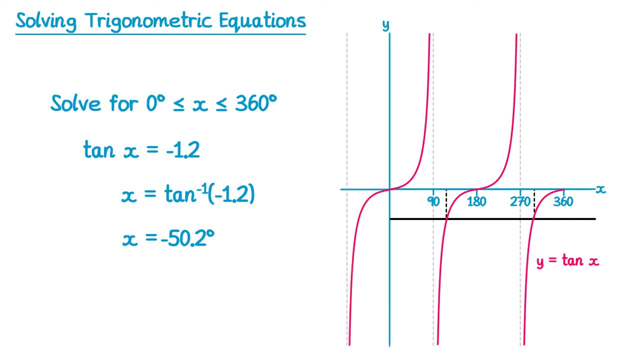 and the graph will go like this. So if we extend our horizontal line backwards, you can see the solution that we've got is here, that's, negative 50.2.. Now, it's a little bit easier than sine, because of this property that it repeats every 180. 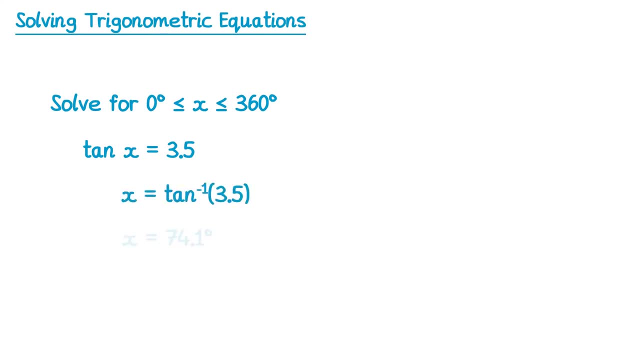 We start in the usual way. We do inverse tan of 3.5 and that gives you 74.1 degrees to one decimal place. Now let's draw the graph of y equals tan of x. You should know that there are two asymptotes on the graph of tan x. You can see those at 90 and 270 degrees and the graph goes like this. 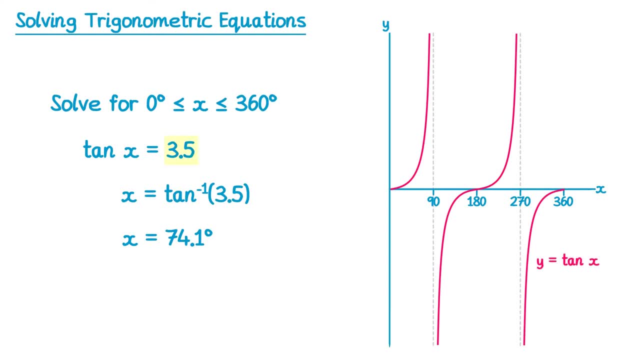 So we're trying to solve this equation equal to 3.5 so we'll draw a horizontal line at 3.5 somewhere about here and we get 2.5. So one of those is our 74.1. That's going to be the left hand solution here and we need to find the right hand solution. Now tan is actually quite nice because tan repeats every 180, not 360 but 180. So we add 180 to 74.1 and we just get the next solution. 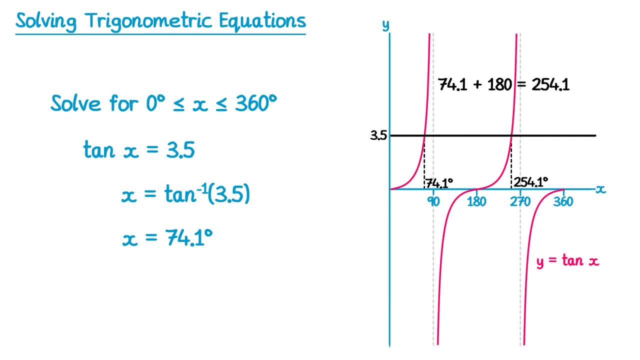 So 74.1 plus 180 is 254.1. So there's our two solutions 74.1 and 254.1 degrees. 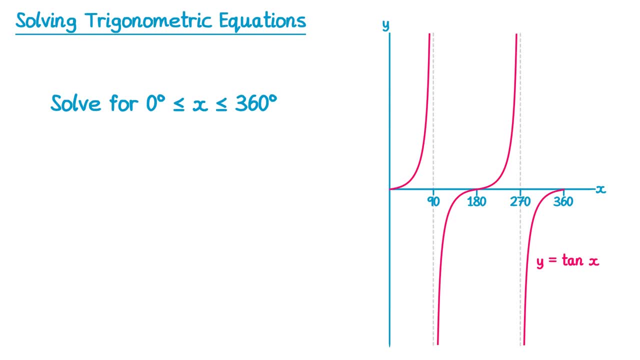 Now like that really nasty equation with sine, if you make tan equal to a negative value we do have a similar problem again. So if we do inverse tan of negative 1.2 we end up with negative 50.2 which isn't in between 0 and 360 degrees. So we need to extend the tan graph backwards as well. So this one was equal to negative 1.2 so we'll draw that horizontal line on first and you can see the two solutions that we're trying to find they're here. Now if we extend the graph backwards we'll have another asymptote at negative 90 degrees. And the graph will go like this. So if we extend our horizontal line backwards you can see the solution that we've got is here. That's negative 50.2. Now it's a little bit easier than sine because of this property that it repeats every 180 degrees. So we just add 180 to negative 50.2 and we get the next one. So that's 129.8 and we add 180 to that one and we get the next one. So 129.8 plus 180 is 309.8. 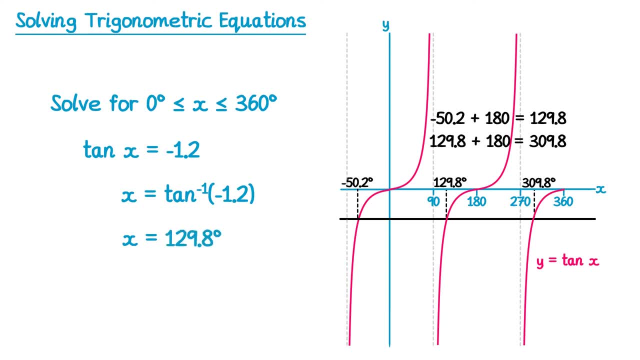 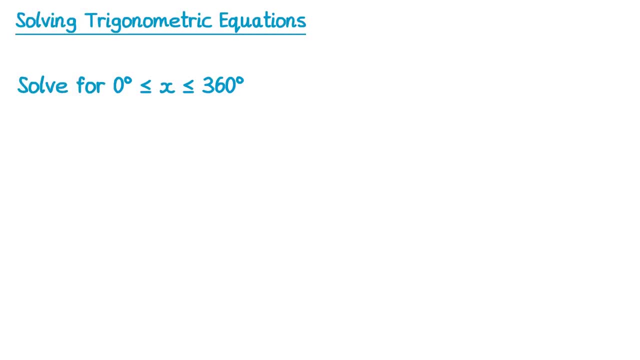 So we don't want that negative solution so we'll lose that and we want our positive 129.8 and 309.8 and they're your solutions. Now those are the basic sorts of equations. Sometimes you 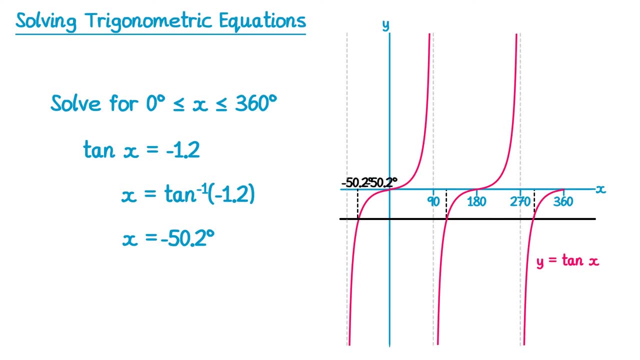 degrees. So we just add 180 to negative 50.2 and we get the next one. So that's 129.8. and we add 180 to that one and we get the next one. So 129.8 plus 180 is. 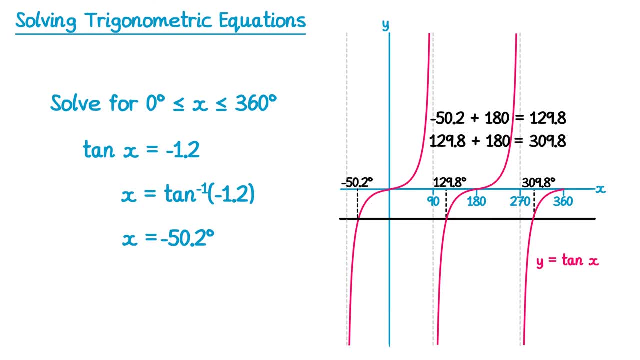 309.8.. So we don't want that negative solution, so we'll lose that, and we want our positive, 129.8 and 309.8, and they're your solutions. Now, those are the basic sorts of equations. sometimes you have to do a bit. 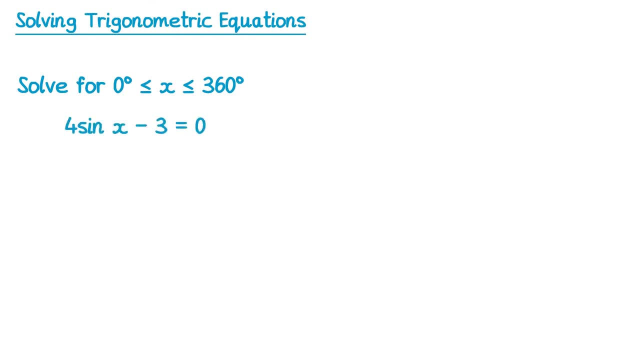 of extra work before you even begin solving. Let's have a look at this equation here. We can only solve this equation when it just says sine x on the left hand side. so we're going to do some rearrangement. Let's add 3 to both sides. 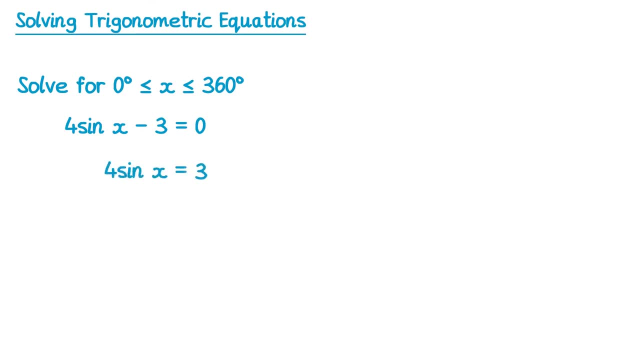 This will give us 4. sine x equals 3.. And then we divide both sides by 4.. If we divide the left by 4, we'll end up with sine x, and if we divide the right by 4, we get 3 divided by 4, which is just. 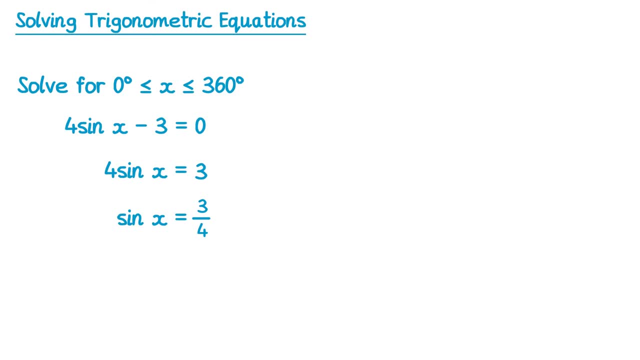 3 quarters. So now we can continue with the question. We do inverse sine of 3 quarters, which gives us our first solution, 48.6, and then we use the graph to get the second one. So let's draw a horizontal line at 3 quarters. that goes: 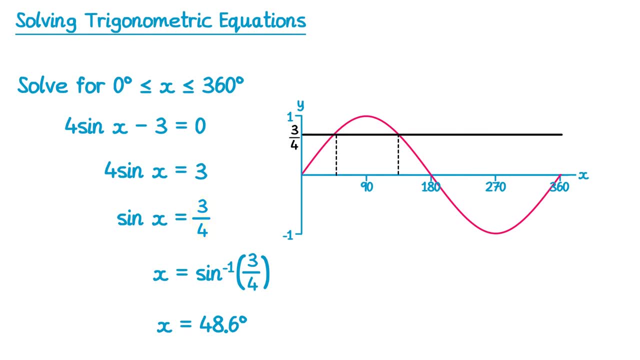 here and we can see the two solutions. The first one: we've got 48.6 and we want this one over here, So we'll use the symmetry of sine here. This distance here is 0 to 48.6, so 48.6. 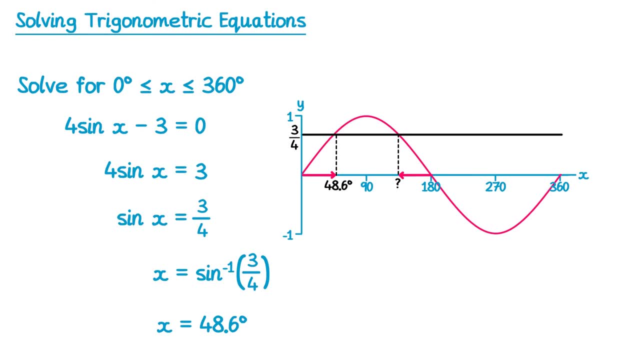 must be the same distance from 180 back to our solution. so 180 take away 48.6 is 131.4 degrees. So we have two solutions to this one: 48.6 and 131.4.. So this one wasn't too much harder. we just had to do some rearrangement. 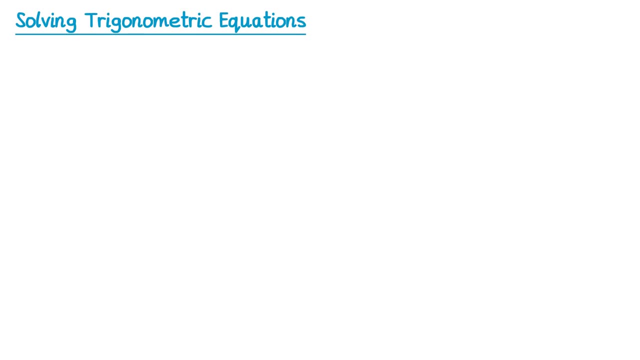 beforehand. Now, before we look at our final type of equation for this video, we need to learn some new notation. Imagine: you started with cos x and you times it by another cos x. This is just the same as cos x squared, because we've timesed it by itself. Now you need to be. 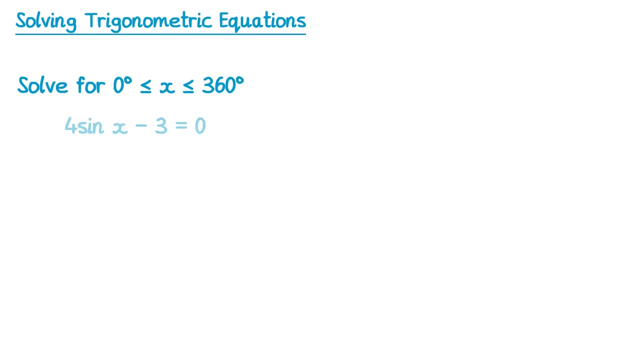 have to do a bit of extra work before you even begin solving. Let's have a look at this equation here. We can only solve this equation when it just says sine x on the left hand side. So we're going to do some rearrangement. Let's add 3 to both sides. This will give us 4 sine x equals 3 and divide both sides by 4. If we divide the left by 4 we'll end up with sine x and if we divide the right by 4 we get 3 divided by 4 which is just 3 quarters. So now we can continue with the question. 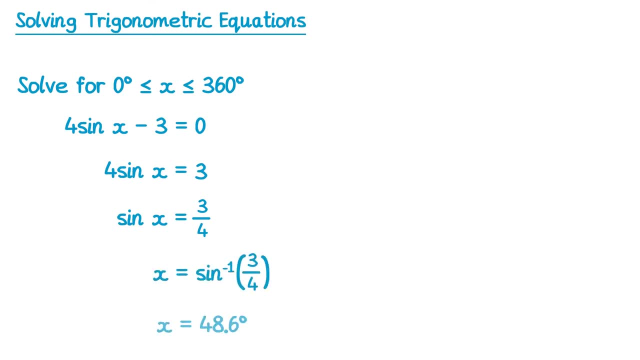 We do inverse sine of 3 quarters which gives us our first solution 48.6 and then we use the graph to get the second one. So let's draw a horizontal line at 3 quarters. That goes here and we can see the two solutions. The first one we've got 48.6 and we want this one over here. So we'll use the symmetry of sine here. This distance here is 0 to 48.6 so 48.6 must be the same distance from 180 back to our solution. So 180 take away 48.6 is 131.4 degrees. So we have two solutions to this one 48.6 and 131.4. So this one wasn't too much harder we just had to do some rearrangement 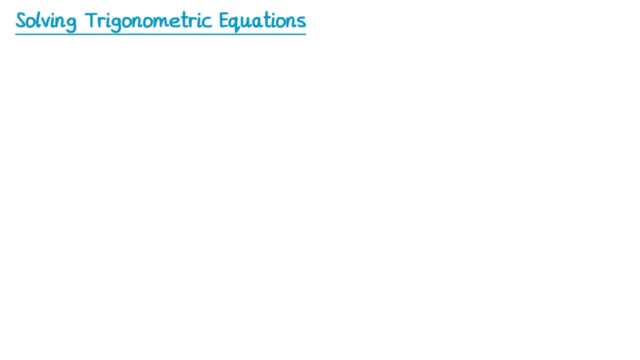 beforehand. Now before we look at our final type of equation for this video we need to learn some 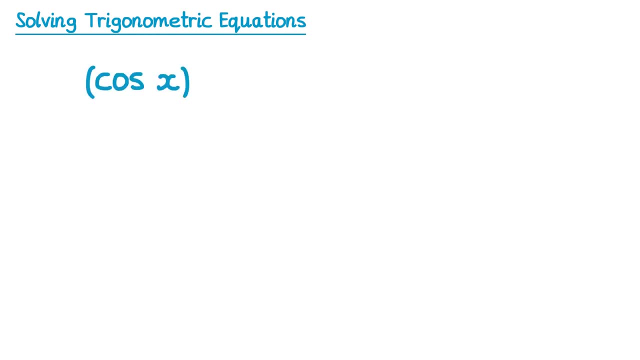 new notation. Imagine you started with cos x. And you times it by another cos x. This is just the same as cos x squared because we've times it by itself. Now you need to be really careful how we write down things in mathematics especially when we have functions like this. If you didn't write the brackets for example and it looked like this, this would be confusing. Does it mean cos x all squared like we've done or does it actually mean cos of x squared where you take a value square it and then do cos of it. It's not necessarily clear. So what we do when we have cos of x in a bracket all squared is we move the squared over here. You would read this as cos squared x. It just means do cos x and then square the result that you get. You can also have sin squared x which is sin x times sin x and tan squared x which is tan x times tan x. It's just easier to write it out in this form. 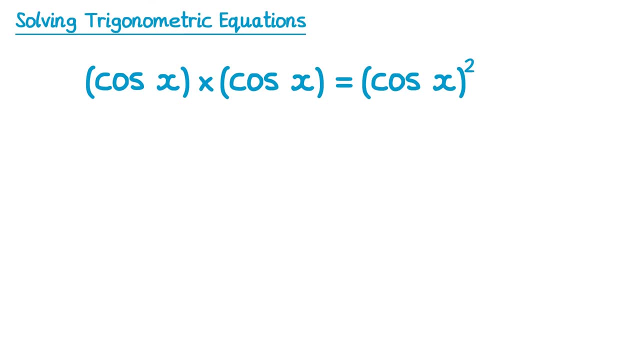 really careful how we write down things in mathematics, especially when we have functions like this. If you didn't write the brackets, for example, and it looked like this, this would be confusing. Does it mean cos x all squared, like we've done, or does it actually mean cos of x squared, where you take a value, square it? 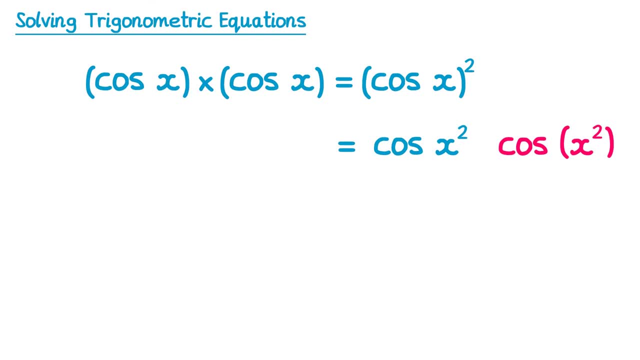 and then do cos of it. It's not necessarily clear. so what we do when we have cos and then square it, is to put a fraction of x on the square. We do the same thing with cos, x squared and then do cos of x. 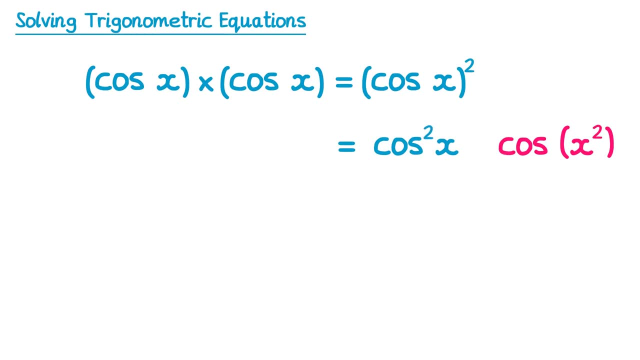 of x in a bracket. all squared is we move the squared over here. You would read this as cos squared x. It just means do cos x and then square the result that you get. You can also have sine squared x, which is sine x times sine x, and tan squared x, which is tan x times tan x. It's just. 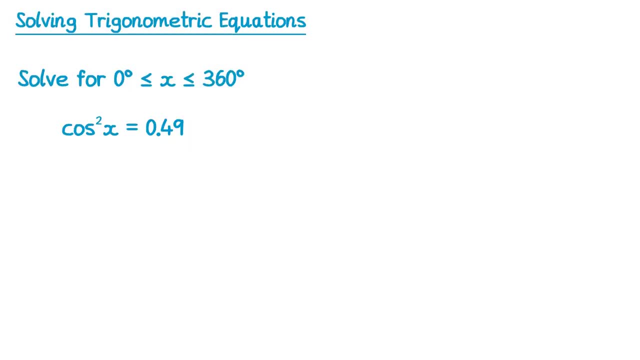 easier to write it out in this form. So let's have a look at an equation with cos squared, x in it. So remember, the left hand side is just cos of x all squared. So the first thing we're going to do is square root both sides of this equation. If we square root the left hand side, we'll lose. 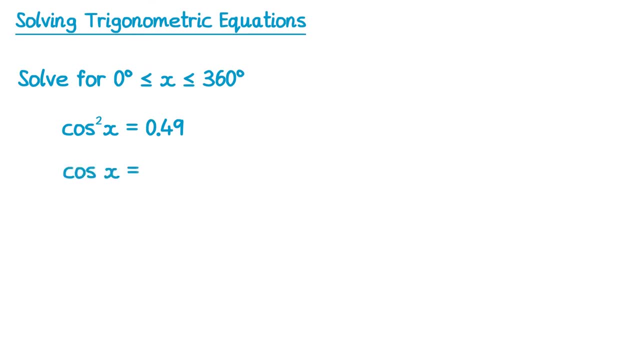 the squared, so we just get cos x, And if we square root the right hand side, we need to do the positive and negative versions of this. so it's plus or minus 0.7. So we need to solve: cos x equals 0.7 and also cos x equals negative 0.7.. So we've got two things to do here, So we'll start with. 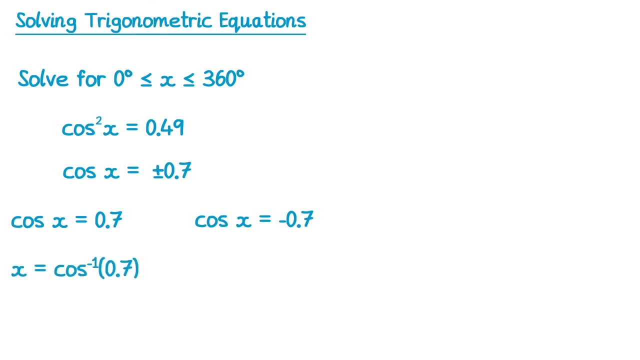 the left hand one, Let's do inverse cos of 0.7, which gives you 45.6 degrees, and then plus or minus 0.7, which gives you 45.6 degrees. For the right one, we'll do inverse cos of negative 0.7, which gives you 134.4 degrees. 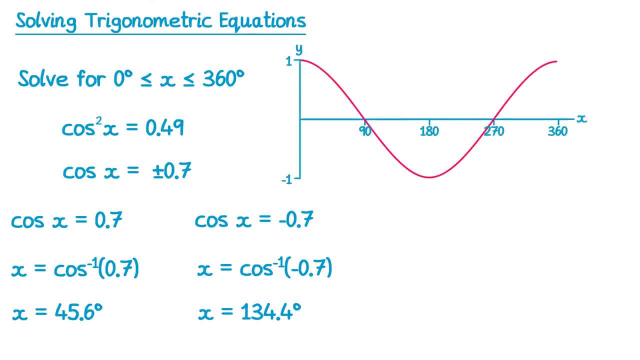 Now to find the other solutions. we're going to use the graph. So if we focus on the left one, when cos x equals 0.7, we draw a line at 0.7 and we'll get two solutions. We already have one of those- 45.6- and we need the other one, So we'll use the symmetry. 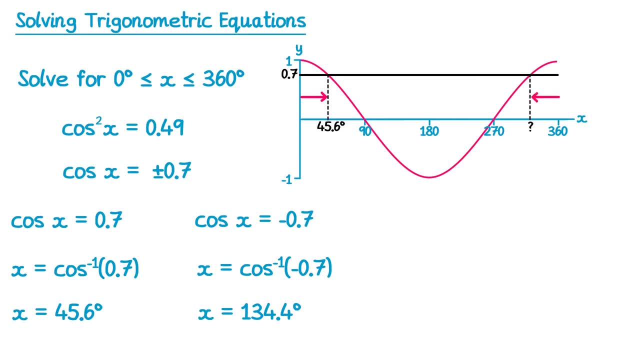 If this is 45.6 degrees, we just take that from 360, and that gives us the other solution: 314.4 degrees. So we found another one, and now if we look at cos x equals negative 0.7. we need to draw that line on as well. That gives us two solutions too. We've already got one of those. 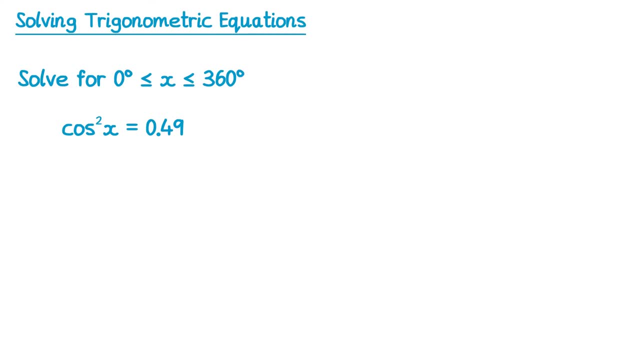 So let's have a look at an equation with cos squared x in it. So remember the left hand side is just cos of x all squared. So the first thing we're going to do is square root both sides of it. If we square root the left hand side we'll lose the squared so we just get cos x. And if we square root the right hand side we need to do the positive and negative versions of this so it's plus or minus 0.7. So we need to solve cos x equals 0.7 and also cos x equals negative 0.7. 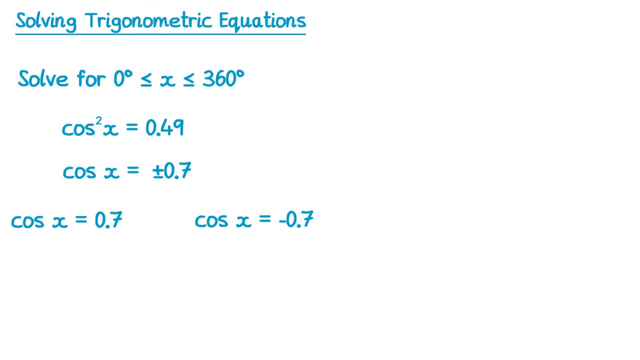 So we've got two things to do here. So we'll start with the left hand one. Let's do inverse cos of 0.7 which gives you 45.6 degrees and then for the right one we'll do inverse cos of negative 0.7 and then for the right one we'll do inverse cos of negative 0.7. Which gives you 134.4 degrees. Now to find the other solutions we're going to use the graph. 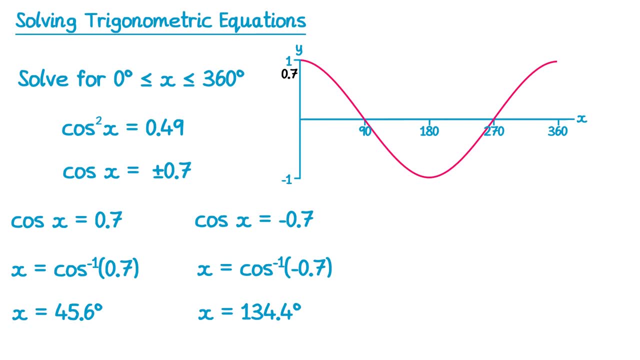 So if we focus on the left one when cos x equals 0.7 we draw a line at 0.7 and we'll get two solutions. We already have one of those 45.6 and we need the other one. So we'll use the symmetry. 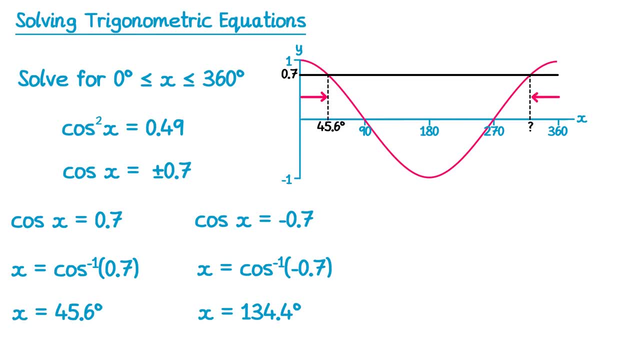 If this is 45.6 degrees we just take that from 360 and that gives us the other solution 314.4 degrees. So we found another one. 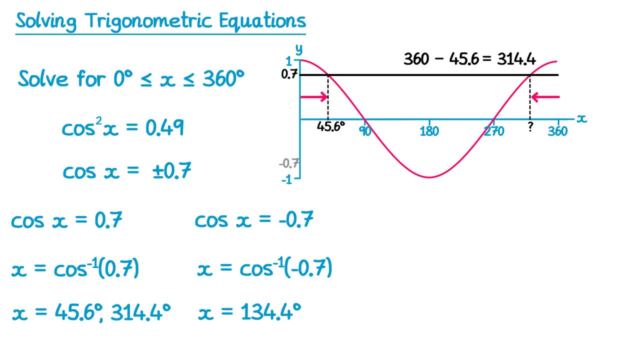 And now if we look at cos x equals negative 0.7 we need to draw that line on as well. That gives us two solutions too. We've already got one of those that's 134.4 and we need this one on the right here. So again we use the symmetry of the graph this is 134.4. 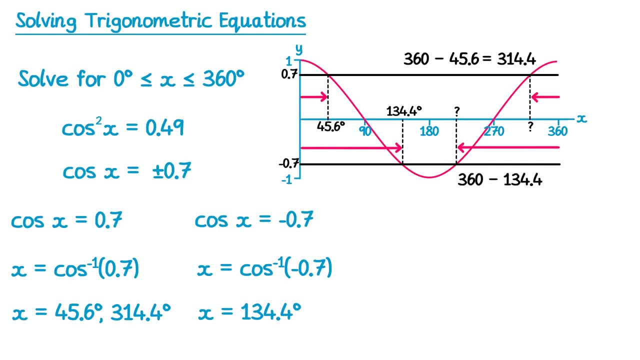 This must also be the same distance so we do 360 take away 134.4 and we get the other solution 225.6. So for this equation there are actually four solutions between 0 and 360. 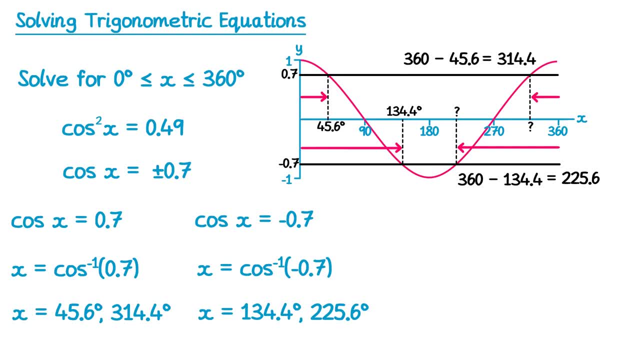 We normally write them out in numerical order so we have the lowest one 45.6, 134.4, 225.6 and 314.4 degrees. 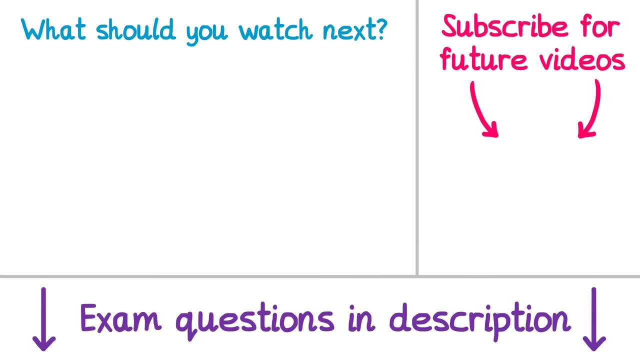 Thank you for watching this video. I hope you found it useful. Remember there are some exam questions in this video's description. Check out the video I think you should watch next and subscribe so you don't miss out on future videos. 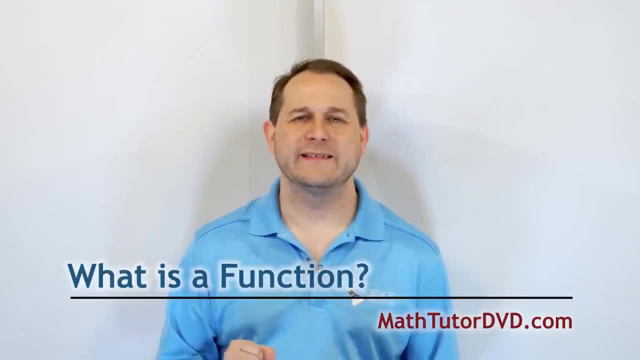 Hello, welcome back to Algebra. In this lesson we're going to cover the concept of what is a function. Now, in the last section we talked about relations and functions in algebra and how they're very similar to one another and how a function is different from a relation. Now we're going to take